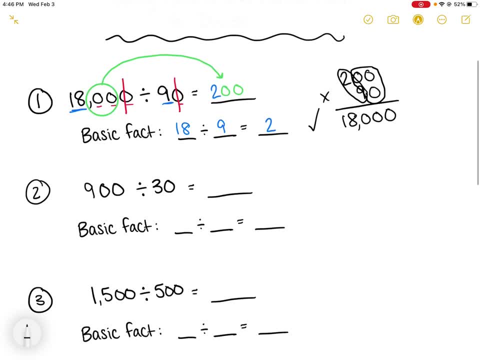 answer is 18,000.. And that's how I know that my answer is correct. Let's try number two. For number two, we have 900 divided by 30. So again, let's use our basic facts of 9 divided by 3. And we know. 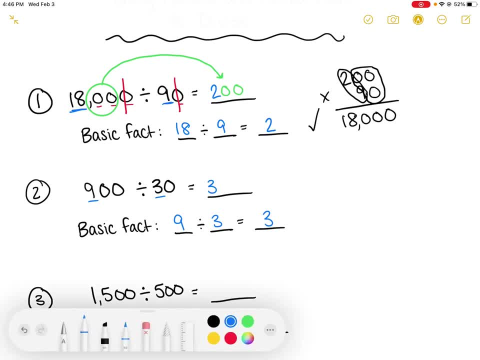 that 9 divided by 3 is 3.. So that's the first part of my answer. And now let's look at our zeros. We have one zero in 30. And two zeros in 900.. So I can definitely cancel out one And I do have one zero left over, So that. 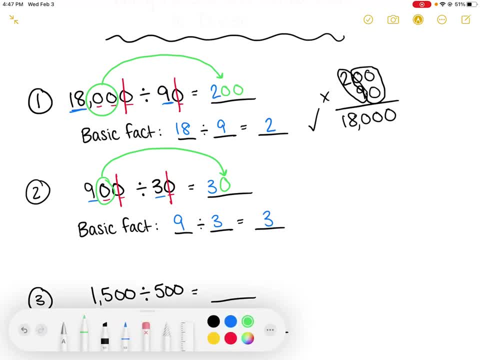 means that one zero left over will get added to my answer, which will be 30.. Now let's check by doing some multiplication. So we'll do 30 times 30. And if we are correct, we should get the answer of 900. 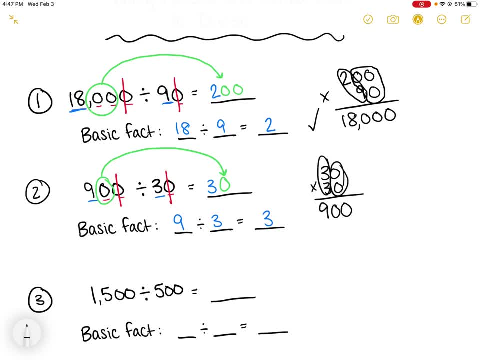 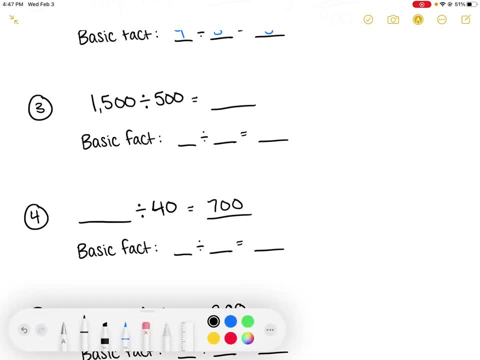 So I know that 3 times 3 is 9. And I have two zeros left over. So yes, 900 divided by 30 does equal 30.. Now let's move on to number three. For number three, we have 1,500 divided by 500.. So let's. 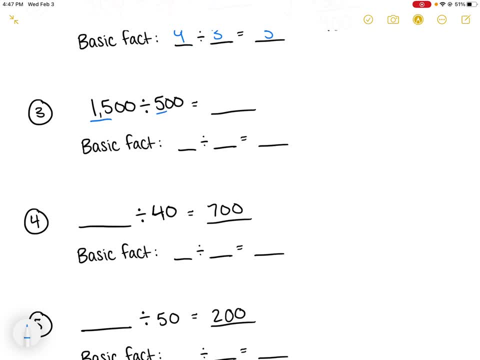 first use our basic facts. So we have 15 divided by 5. And we know that equals 3.. So that's the first part of my answer. Now let's check our zeros. We have two zeros in 500, two zeros in. 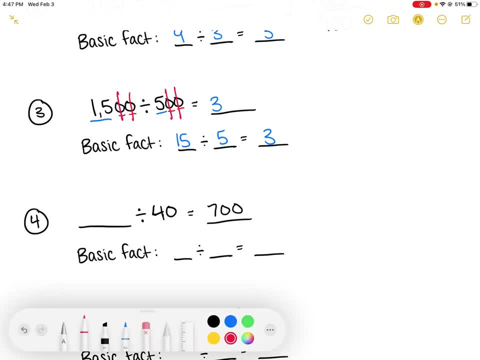 1,500.. So they cancel each other out And there are no zeros left over. So that means that our answer is just 3.. So let's double check with some multiplication just to make sure that we're correct. So we have to do. 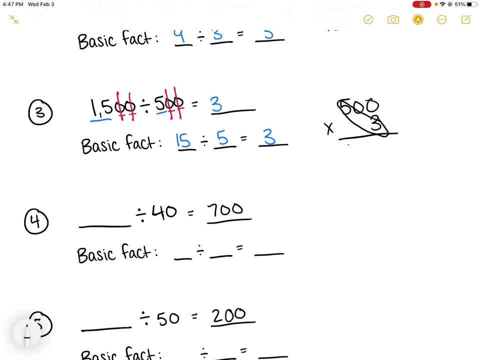 500 times 3.. I know that 5 times 3 is 15.. And there's two zeros left over, So 1,500.. And our answer is correct. Now let's go to number four. These are a little different. They give you the. 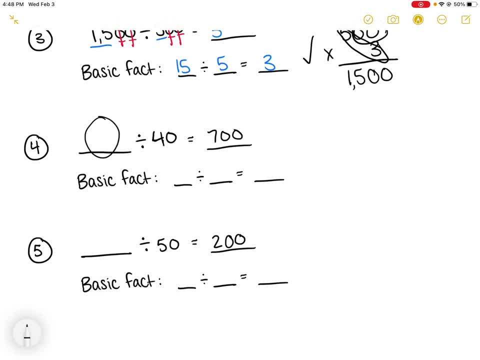 answer, but we are looking for a missing number here. So we have something divided by 40 equals 700.. So I still want you to think about your basic facts. So we will have something divided by 4 equals 7.. Now, in order to find our answer, what we can do is do the opposite of division, which is 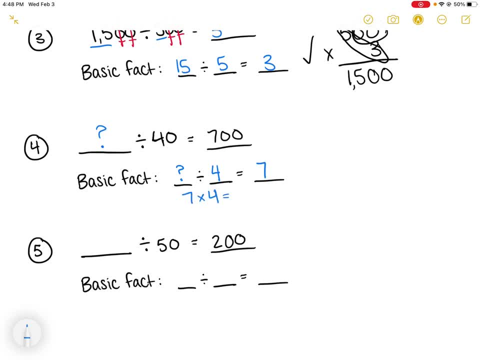 multiplication, We can do 7 times 4. And that will give us 28.. So we know that our missing factor for our basic problem should be 28.. Now what we have to do is figure out how many zeros are next to that 28.. Well, let's see, Let's think. 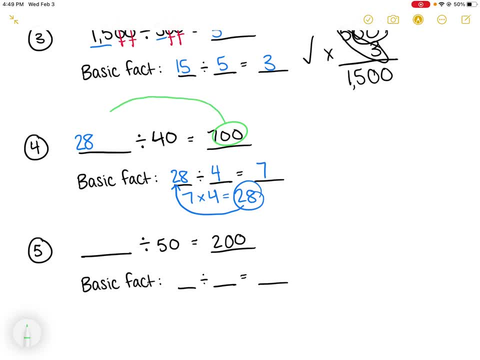 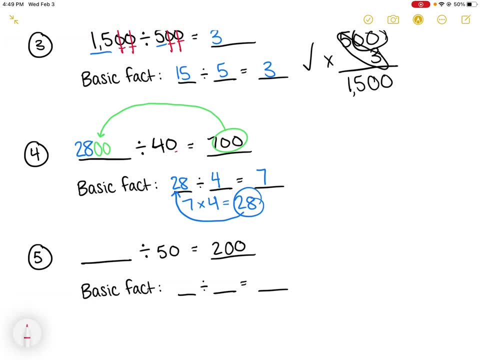 backwards. We have two zeros in our answer, So that means there was two zeros left over when we were dividing. And we also know that there is one zero in 40. So that means one zero got cancelled out. So our answer to the missing number is that it is 28.. 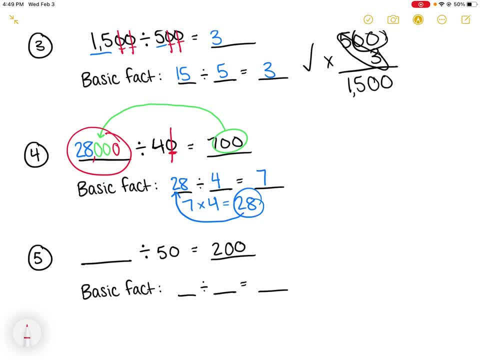 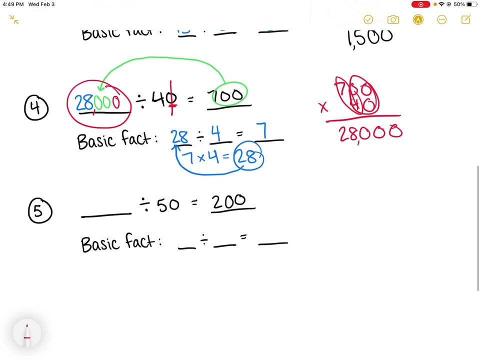 Now again, you can double check this by doing some basic multiplication. You can do 700 times 40.. 7 times 4 is 28.. And we have three zeros, So it's 28,000.. And then, last, let's go to number. 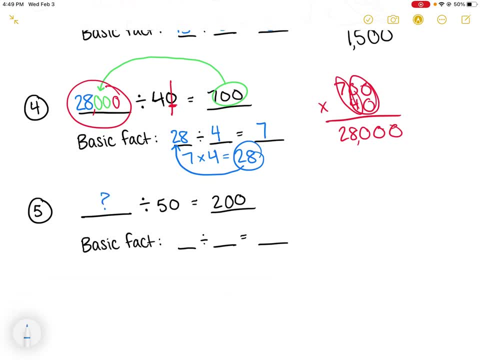 five. So number five is: something divided by 50 equals 200.. So let's think to ourselves: Something divided by 5 equals 2.. so I'm going to use multiplication. so 2 times 5 gives me 10. so 10 is my missing. 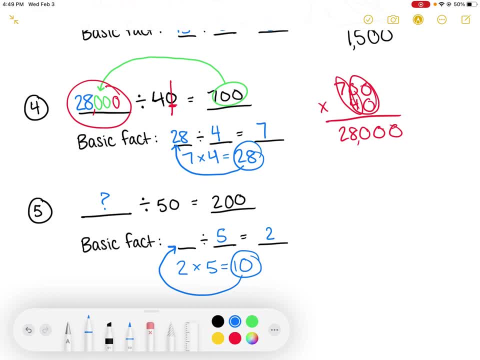 number up here, and I know that 10 is part of my missing number up on top here as well, remember, you have to figure out now how many zeros do I need. well, I know that there are two zeros left over, and then one zero got cancelled out, so that 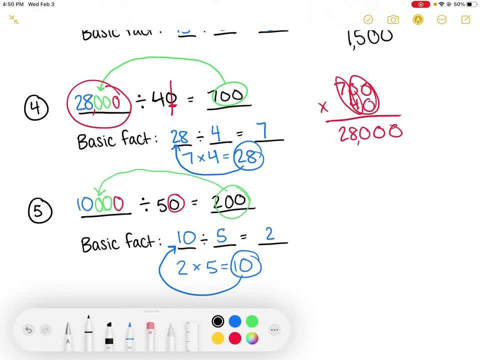 means I have to add one extra zero, so my answer should be 10,000. we can check this by again doing some multiplication. we can do 200 times 50, so we have 5 times 2, which is 10, 3 zeros. so 10,000. that's what we got before. this is how. 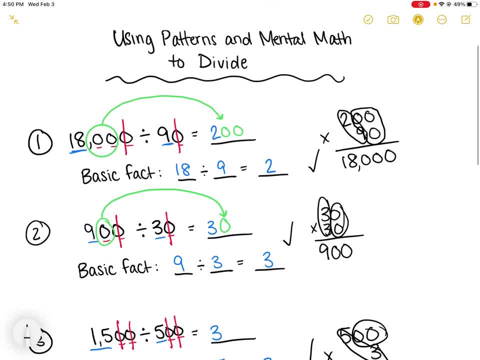 you can use patterns and mental math to find division problems.